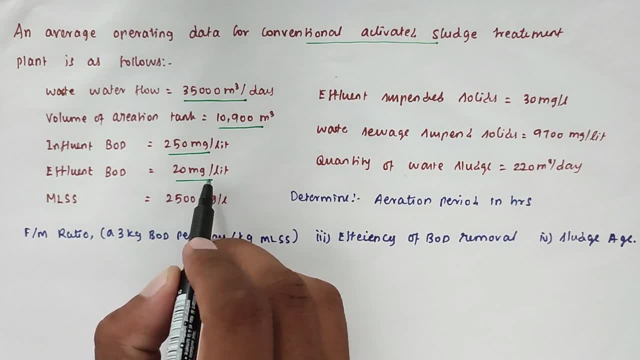 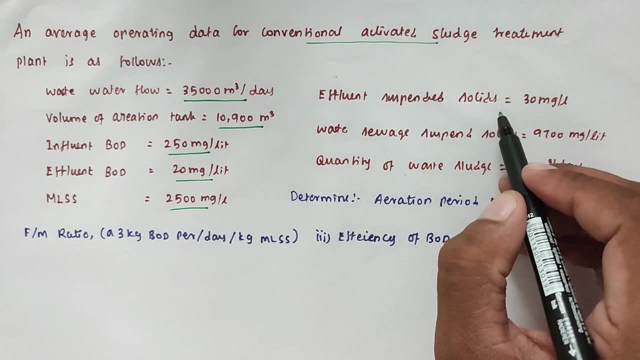 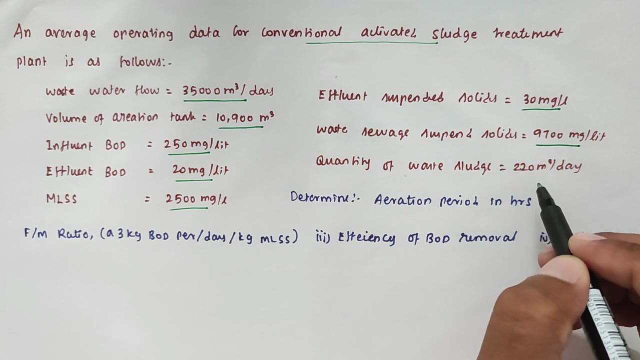 BOD: 250 milligram per liter. effluent BOD: 20 milligram per liter. MLSS: 2500 milligram per liter. then effluent suspended solids is 30 milligram per liter, waste sewage suspended solids: 9700 milligram per liter. then quantity of waste sludge is 220 milligram meter cube per day. okay so. 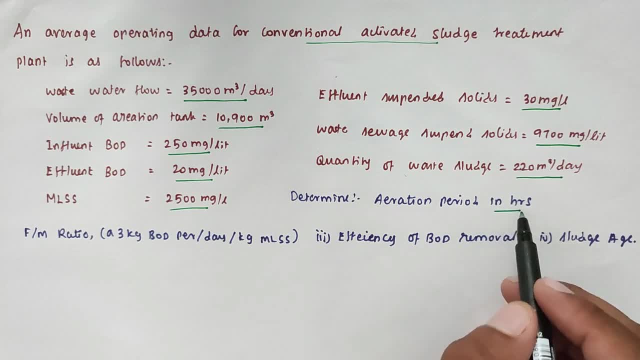 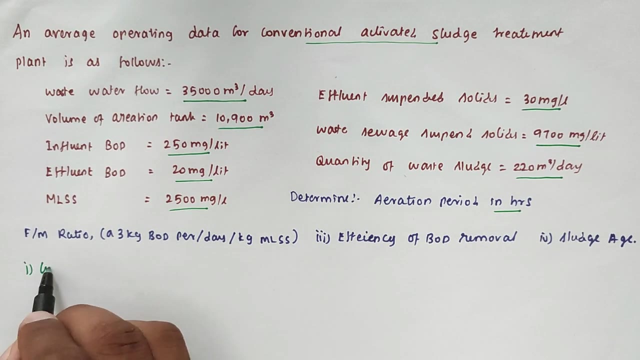 we have to find out: determine aeration period in hours, then FM ratio by foot, by microbial mass ratio, then efficiency of BOD removal, then sludge age. okay, so these are all the things we have to find out. so first thing is: given value, so given the Q. 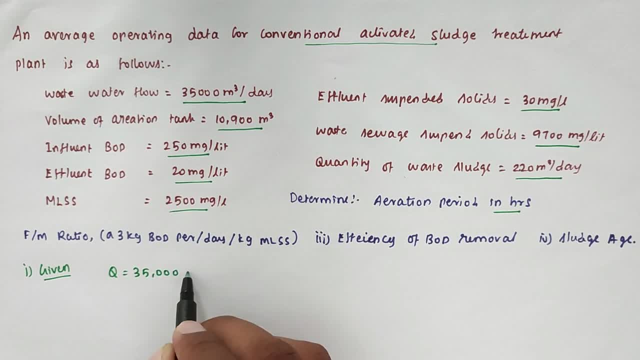 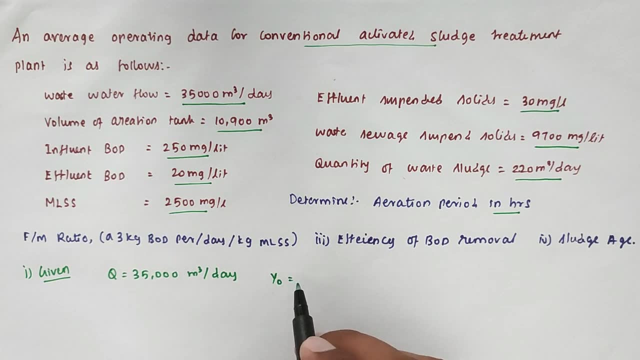 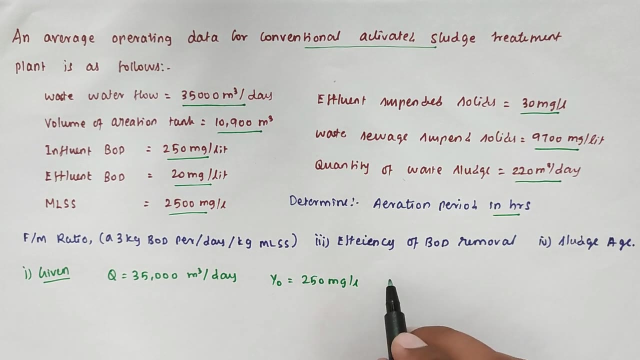 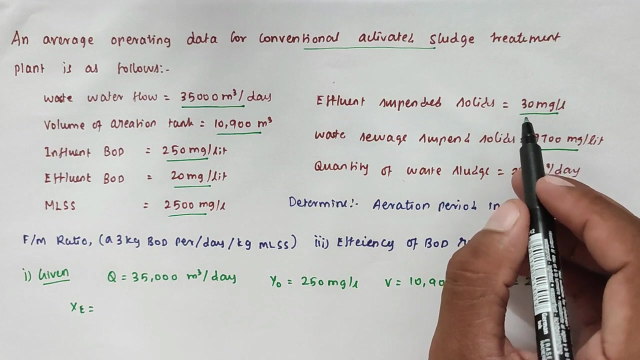 value is 35,000 m cube per day. so then why not? so that is a influent BOD is 250 milligram per liter, Then volume of aeration tank V, equal to 10900 m3.. So then Xt, that is MLSS, that is 2500 mg per litre. Then Xe is effluent suspended solids, that is 30 mg per litre. 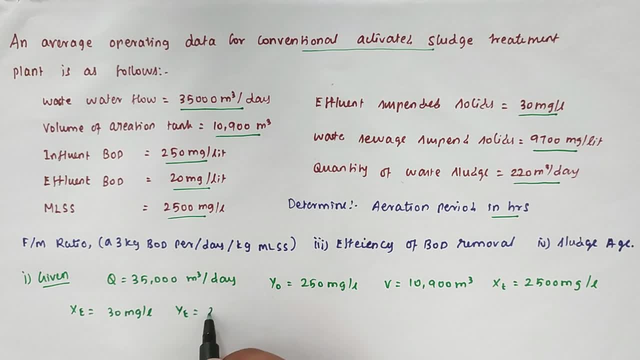 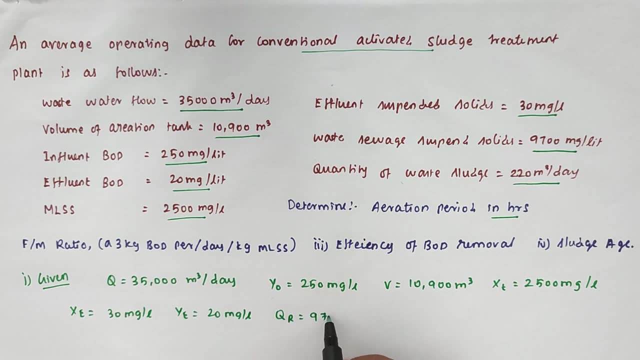 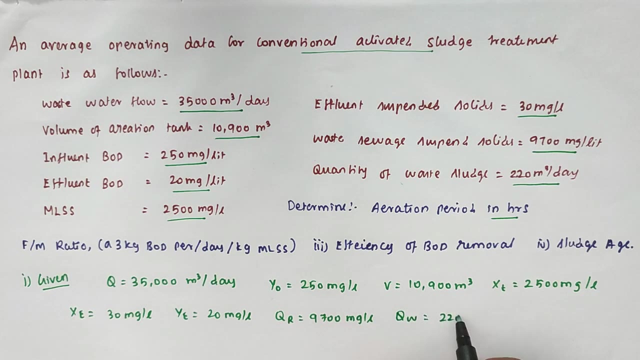 Then Ye, that is effluent BOD is 20 mg per litre, Then Qr, equal to 9700 mg per litre, Then Qw, equal to 220 m3 per day. So these are all the things they are given. So we have to find out. first thing, we have to find out the aeration period in 24 hours. 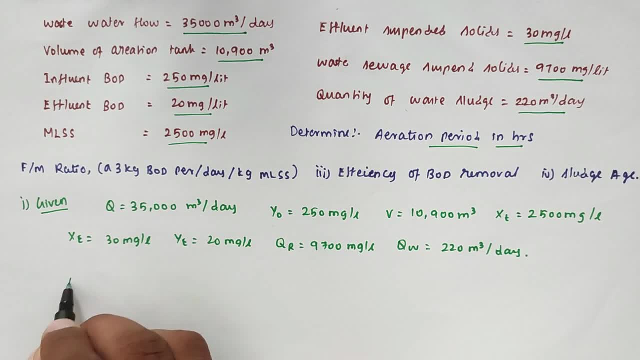 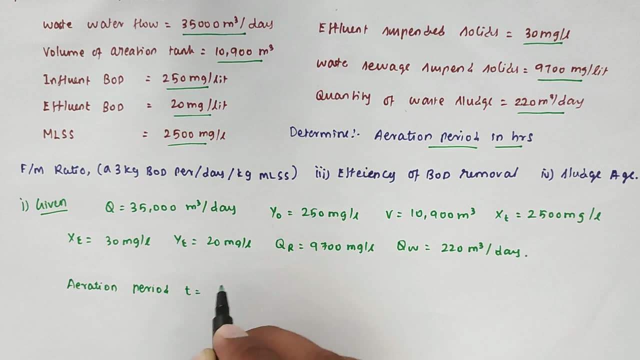 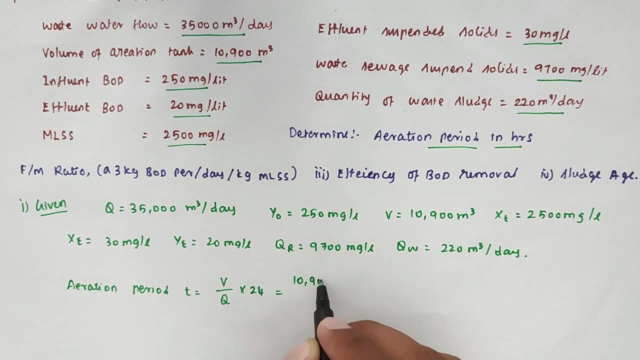 So the formulas for aeration period: Aeration period T equal to V, by Q into 24 hours. Ok, so now we can take 10900 divided by 35000 into 24 hours, So we got the value of 7.47, that is, 24 hours. 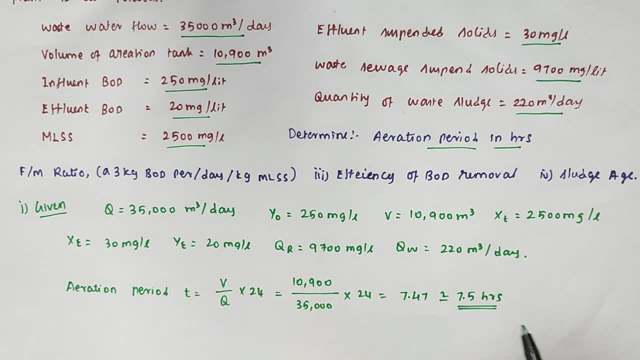 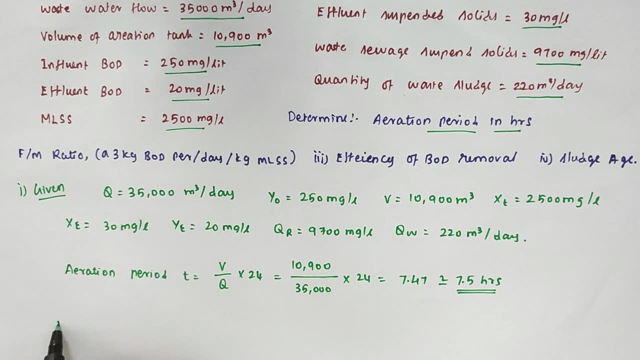 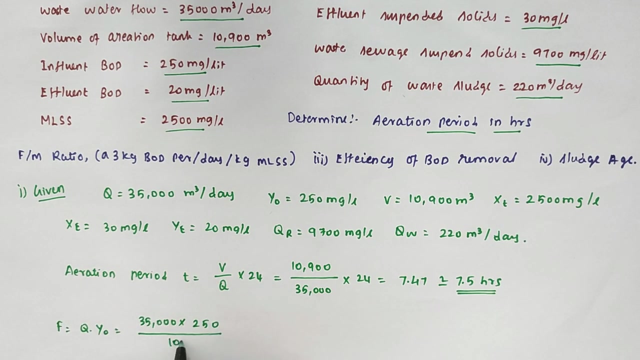 So this is the first question answer. Second thing is foot by micro wheel ratio. So then F equal to Q into Y0, that is 35000 into 250.. So we can convert into kg per day, So we can put 1000. 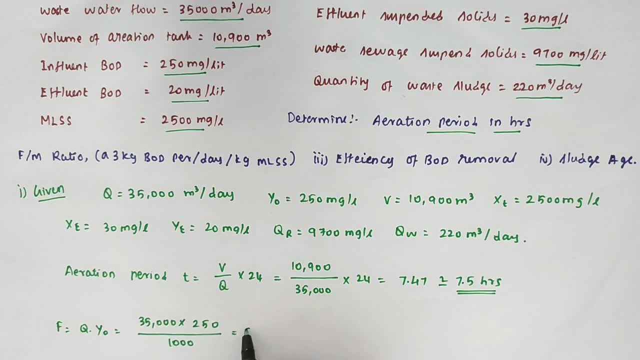 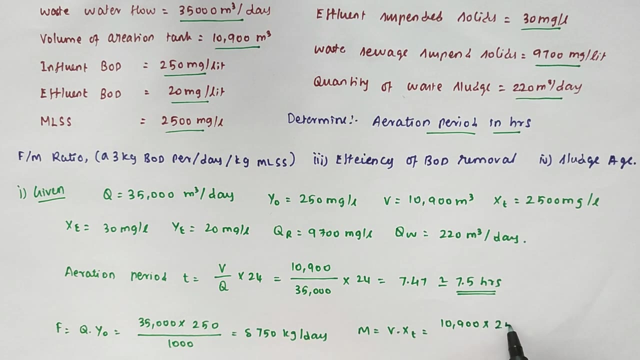 So 1000 kg is equal to 1 mm cube, So that is 8000.. So that is 8750 kg per day. Ok, likewise we can calculate the M value. So M equal to V into Xt, that is V equal to 10900 into Xt value is again 2500 divided by we can convert into kg. 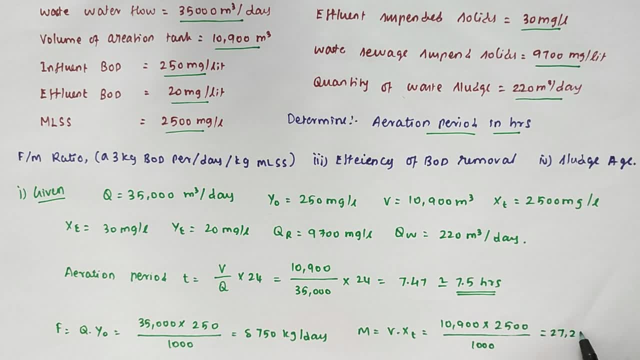 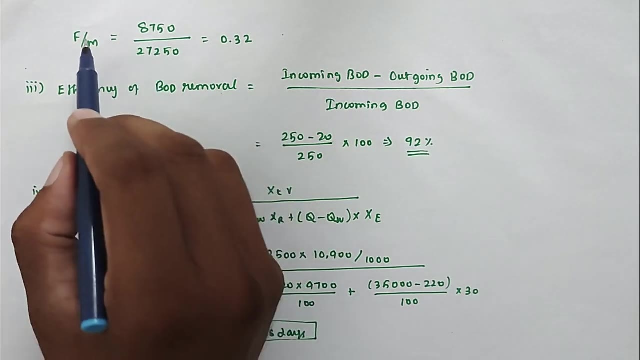 So divided by 1000, equal to 27250 kg. Ok, So now we can easily find out the foot by micro wheel ratio, That is F by M ratio. So now foot by micro wheel ratio. So now F by M. So F, we found out 8750. 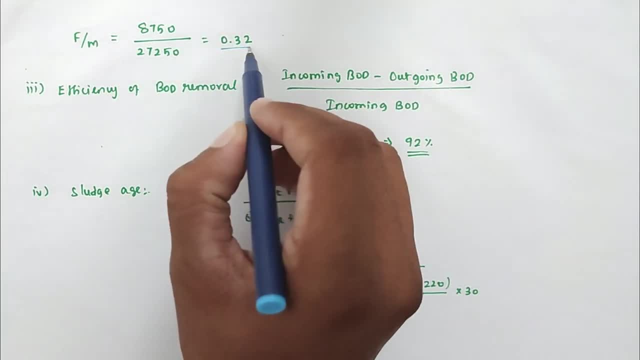 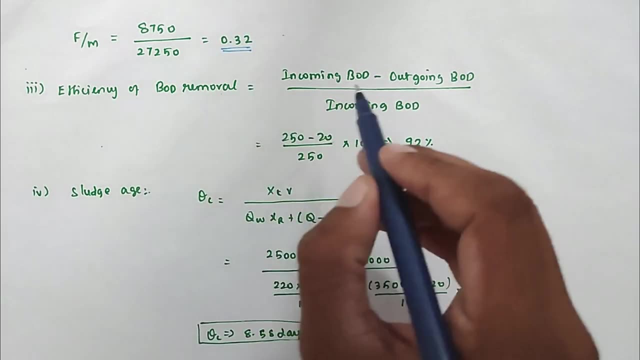 Then M 27250.. So, solving this, we got the value 0.32.. Ok, So, third question: efficiency of BOD removal. So now the formula is incoming BOD minus outgoing BOD divided by incoming BOD. So incoming BOD is 250. 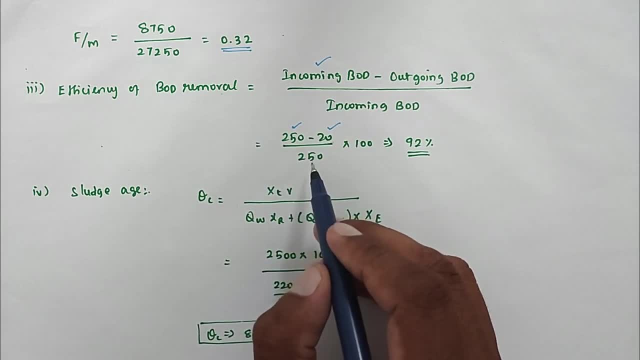 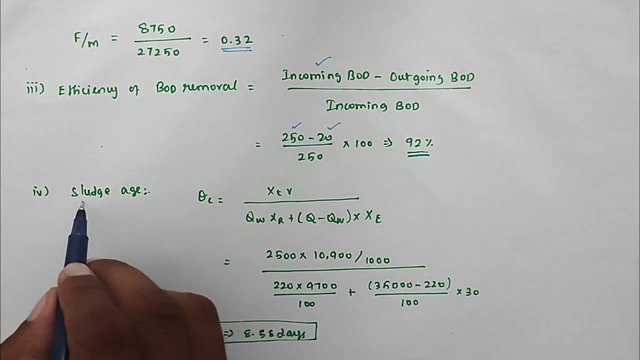 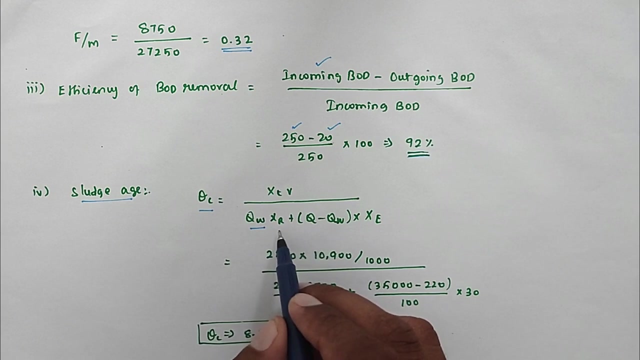 And outgoing BOD is 20.. So 250 minus 20 divided by 250 into 100. So now we got the value of 92 percentage. So fourth question is sludge age. So we know the formula theta C equal to Xt into V, divided by Qw into Xr, plus Q, minus Qw into Xc. 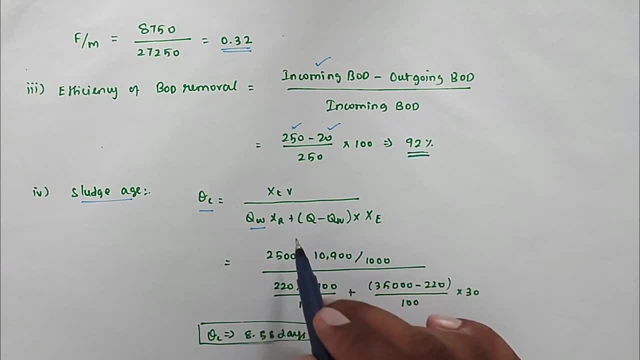 Ok, So now we know all the values. So now we can substitute all the values over here. So Xt equal to 2500, that is given Into the volume, is 10900 divided by 1000.. So divided by Qw, 220 into 9700. divided by 100 plus the Q value, is 35000.